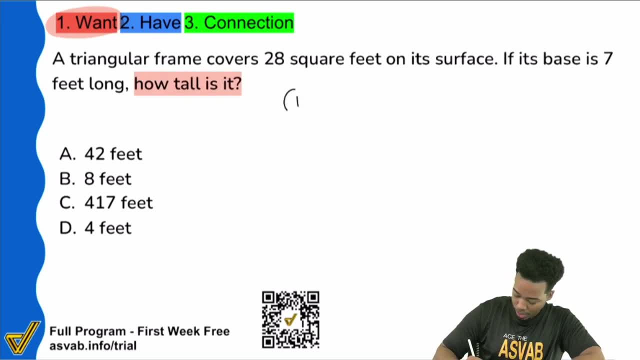 feet long. how tall is it So? okay, cool. It's safe to say that we're looking for some sort of height, So we can say blank Feet tall And again it's probably labeled as some sort of height. Now you want to think in. 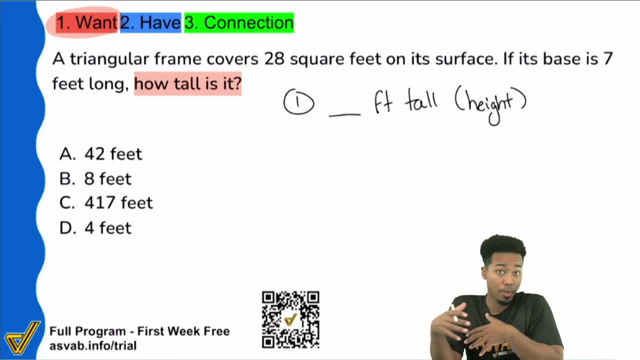 this way because, remember, if you're talking about geometry, times are going to tell you that you are going to have a base, a height, a length or a width or things like that, And if you can recognize those things being stated in the problem, then you might be able to recognize. 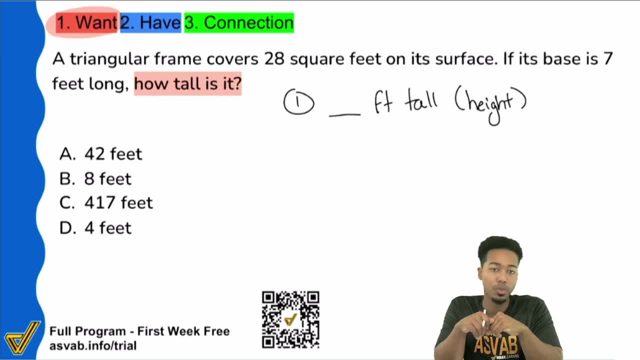 the formula that you might need to use. So, with that said, let's go ahead and get into the information now and see what kind of clues we have to guide us. First things first. I noticed that immediately says hey, a triangular frame. Well, guess what? I? 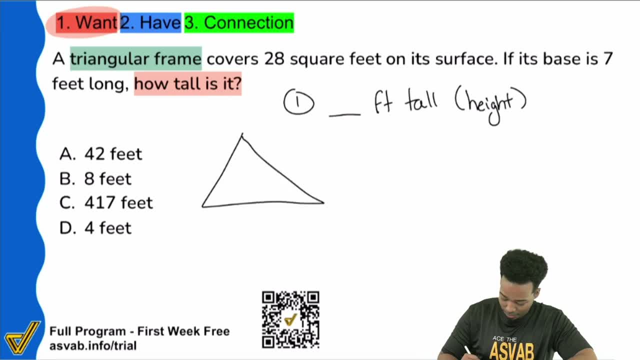 know that we're dealing with a triangle, then. So let me go ahead and draw myself a triangle. Yes, I can draw perfect triangles. Look at that. I can even adjust my drawings in real time, because I'm just Picasso. So, with that said, we have a triangular frame And then this part might be. 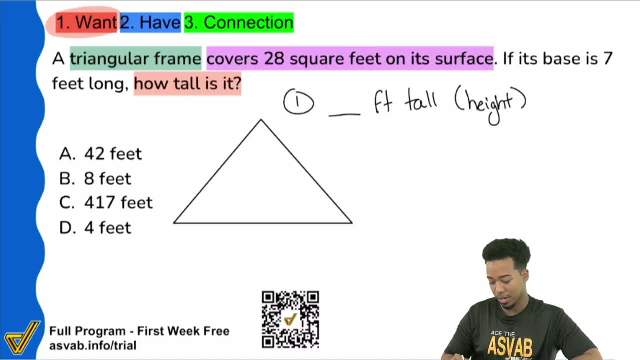 confusing to some of us. It says it covers 28 square feet on its surface. What does that mean? Square feet? Is that perimeter? Is that area, Is that volume? What is that? So this is where, again, when you understand nuance, when you understand the little details, this is going to. 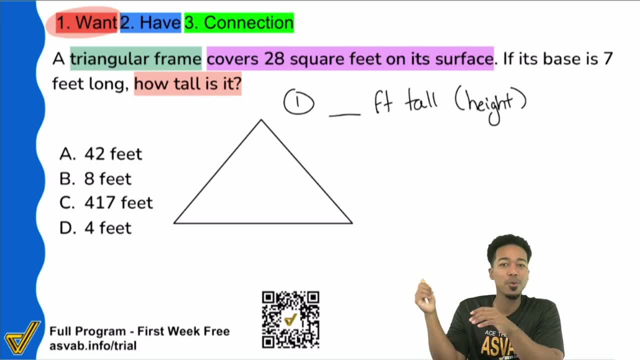 prove to be a huge helper for you. I got you So whenever we're talking about square units- square feet, square inches, square yards, whatever we're talking about area, We are talking about area. Remember that the square in square feet it just denotes that you're dealing with the second. 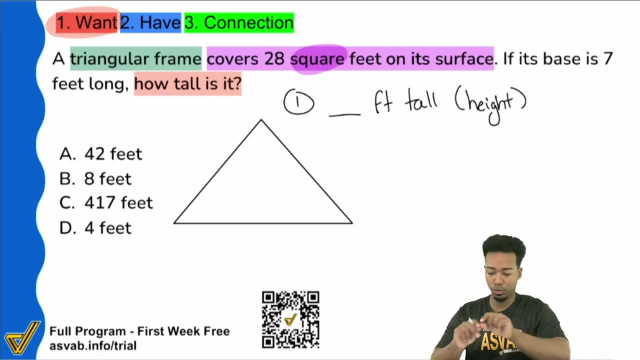 dimension. So if you're saying feet first dimension, So straight line distance, If you say square feet, well that's space, And if you say cubic feet, that's three-dimensional space, because it's the third power. So remember one more time: square feet can be written as feet squared, That's the 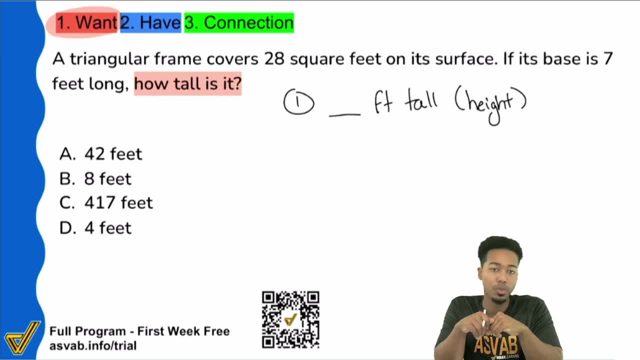 the formula that you might need to use. So, with that said, let's go ahead and get into the information now and see what kind of clues we have to guide us. First things first. I noticed that immediately says hey, a triangular frame. Well, guess what? I? 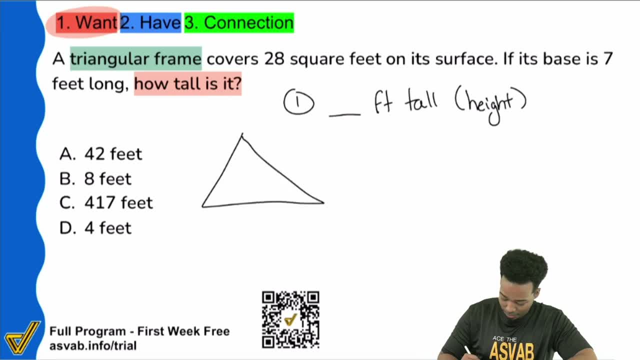 know that we're dealing with a triangle, then. So let me go ahead and draw myself a triangle. Yes, I can draw perfect triangles. Look at that. I can even adjust my drawings in real time, because I'm just Picasso. So, with that said, we have a triangular frame And then this part might be. 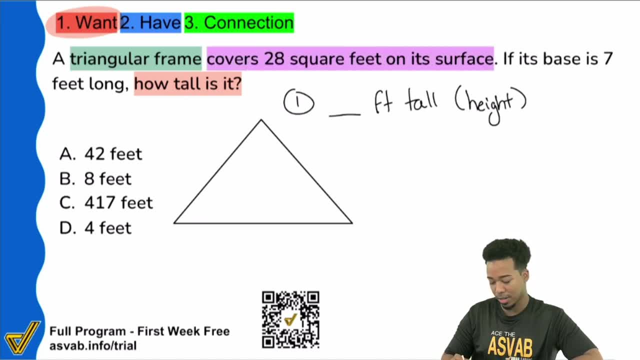 confusing to some of us. It says it covers 28 square feet on its surface. What does that mean? Square feet? Is that perimeter, Is that area, Is that volume Like what is that? So this is where, again, when you understand nuance, when you understand the little details, this is going. 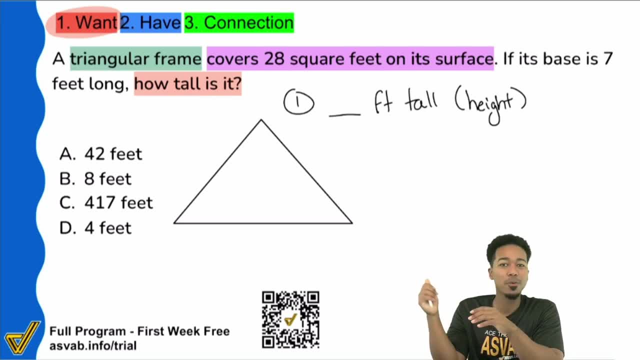 to prove to be a huge helper for you. I got you So whenever we're talking about square units- square feet, square inches, square yards, whatever we're talking about area, We are talking about area. Remember that the square in square feet it just denotes that you're dealing with the second. 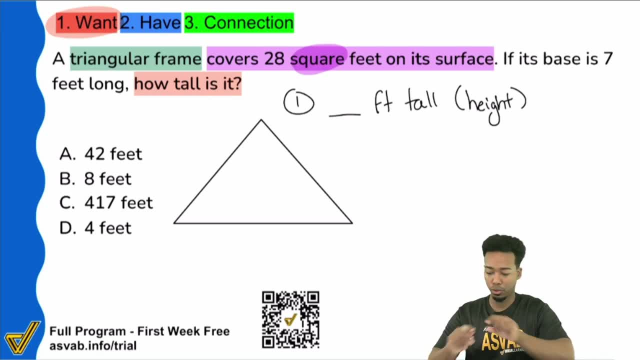 dimension. So if you're saying feet first dimension, So straight line distance, If you say square feet, well that's space, And if you say cubic feet, that's three-dimensional space, because it's the third power. So remember one more time: square feet can be written as feet squared, That's the 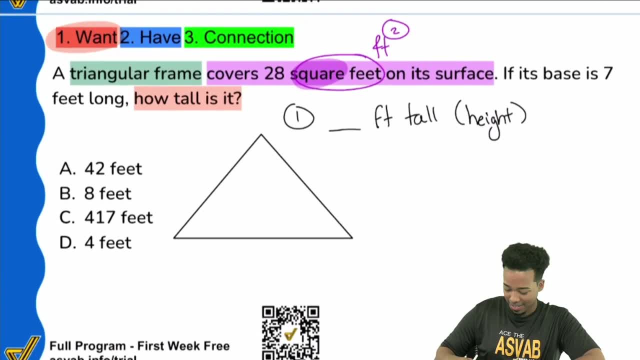 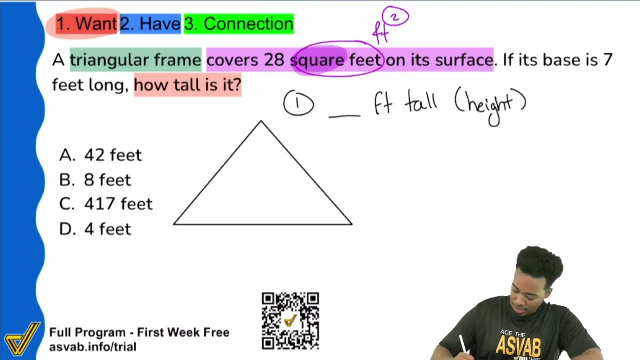 two I'm talking about right there. So, with that said, let me go ahead now and again remind you: 28 square feet. the key here is that that refers to area. So the area of this triangle is the area of the triangle. So that's the area of the triangle, So the area of this triangle. 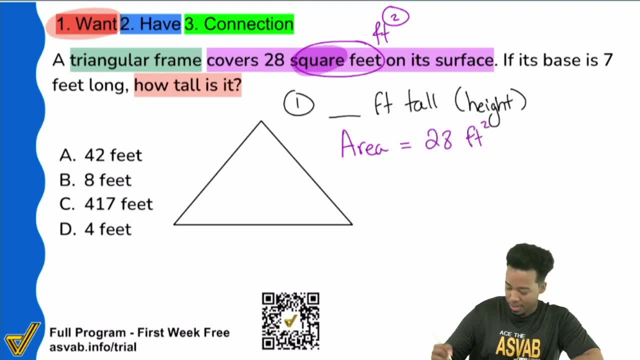 is the area of the triangle, So the area of this triangle is the area of the triangle, So the area of this triangle equals 28 square feet. That's huge for us. huge because the moment that you know you're dealing with something formulaic like perimeter area, surface area, volume, circumference, anything 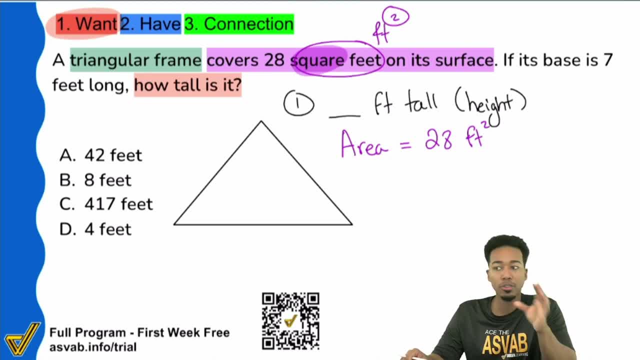 like that. you know that there's a formula associated with it and you should be ready to state that formula whenever needed. So here we're dealing with a triangle and we're dealing with area. So what is the formula? So what is the formula for the area of a triangle? Let me help you out. The area of a triangle. 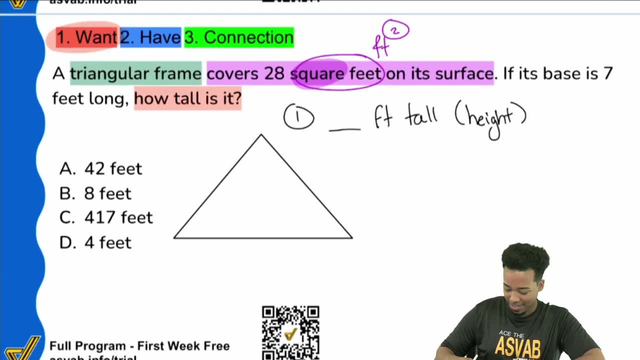 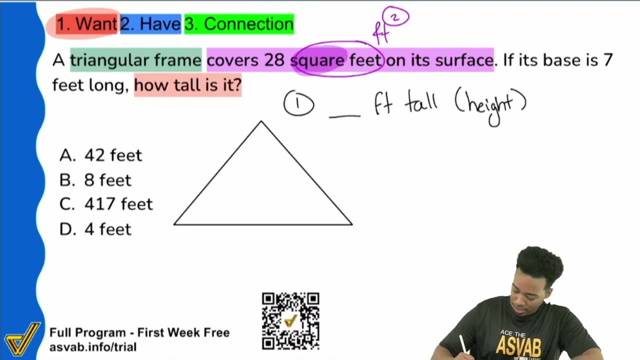 two I'm talking about right there. So, with that said, let me go ahead now and again remind you: 28 square feet. The key here is that that refers to area. So the area of this Triangle, Triangle, Triangle, equals 28 square feet. That's huge for us. Huge Because the moment that you know, 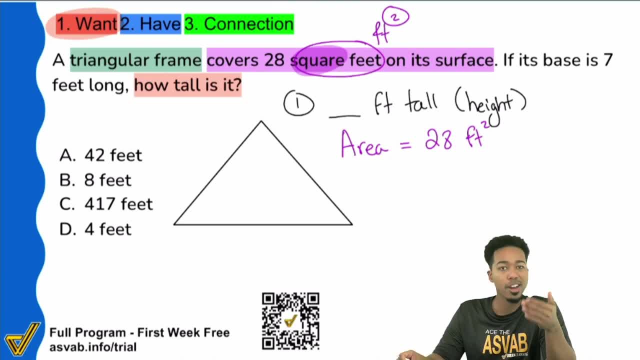 you're dealing with something formulaic like perimeter, area, surface area, volume, you know circumference, anything like that. You know that there's a formula associated with it and you should be ready to state that formula whenever needed. So here we're dealing with a triangle and we're dealing with area. So what is the formula? 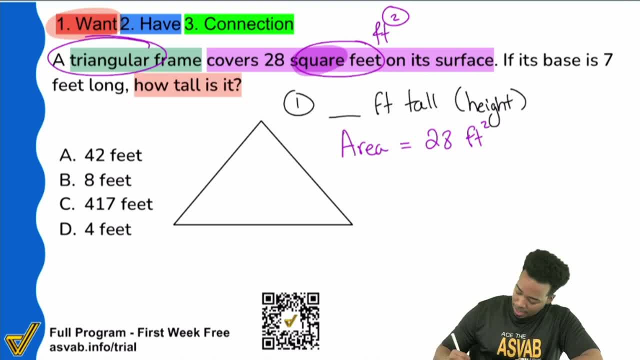 For the area of a triangle. Let me help you out. The area of a triangle is going to be the base times, the height divided by two. That's it right there: Base times, height divided by two. Or you can say one half base times height. 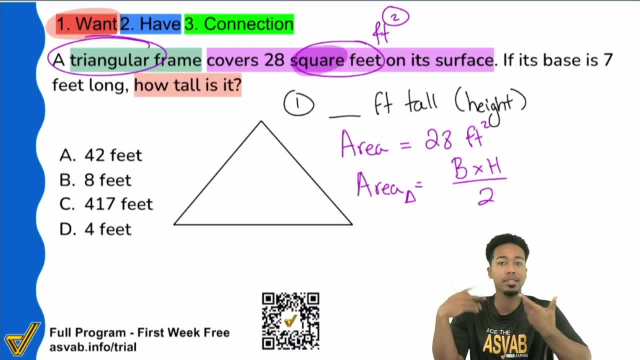 You might know it that way too, but this is the easier way to write it, in my opinion, because it makes it easier to solve the formula for B or H. So, with that said, what else do we know? Well, we also know right over here that we are given 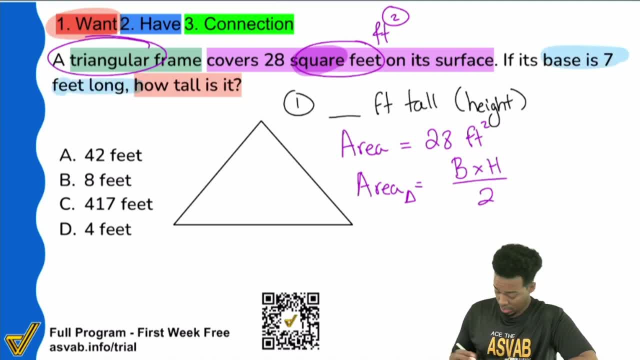 the base as seven feet long. So my base is seven feet long. We want to know how tall it is, So we want to know the height, And we are given the area as, again, 28 square feet. So all we're going to do here is we're. 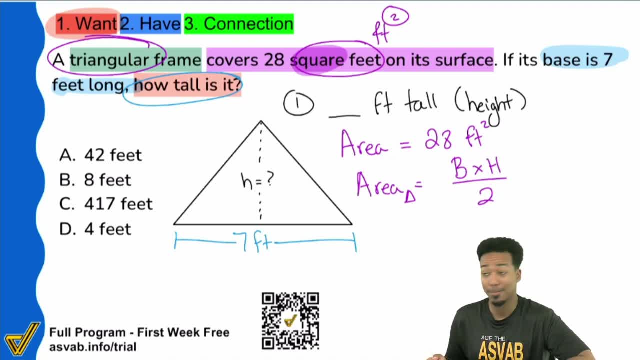 going to plug in the information and we're going to have ourselves a good time. That's it, The area that we're given. my party people remember that was 28.. Then the base that we were given was seven, And then we're looking for the height and then we are filling in the rest of the formula. 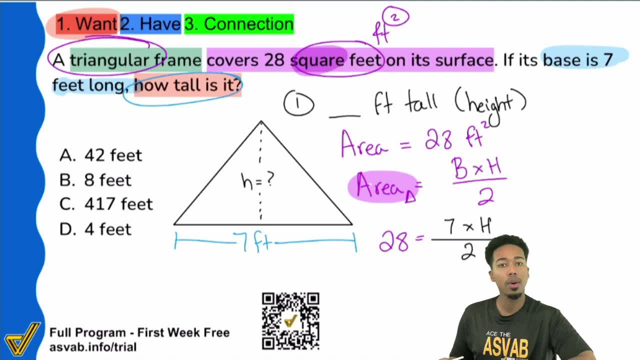 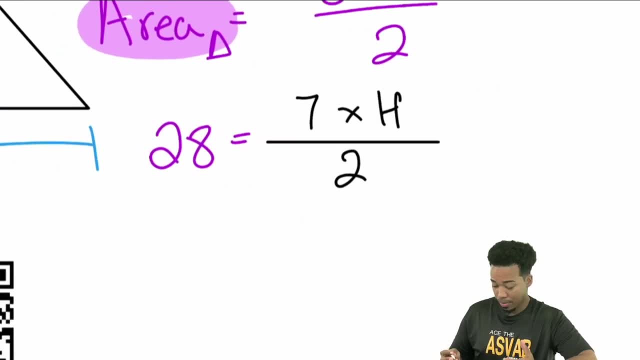 Now all I have to do, my party people, all I got to do is go ahead and solve this equation here, and we're set. Here we go. First things first. I could probably get away with multiplying both sides by two, or you could divide both sides by seven. Either way, you're just trying to get rid of everything. 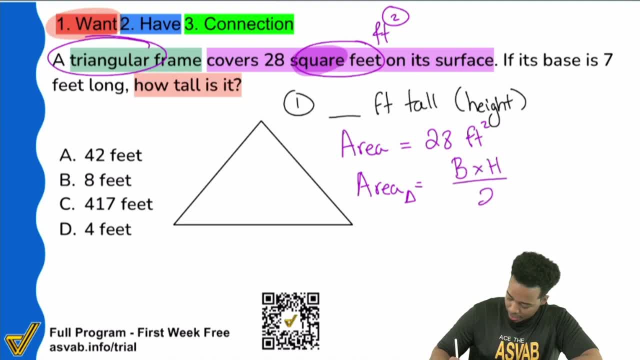 is going to be the base times the height divided by two. That's it right there: Base times height divided by two. Or you can say one half base times height. You might know it that way too, but this is the easier way to write it, in my opinion, because it makes it easier to solve. 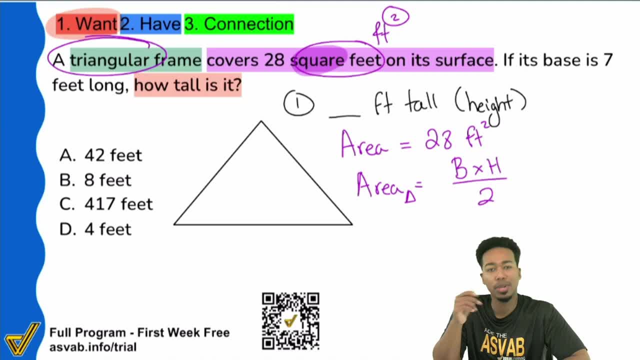 the formula for B or H. So, with that said, what else do we know? Well, we also know, right over here, that we are given the base as seven feet long. So my base is seven feet long. We want to know how tall it is, So we want to know the height. 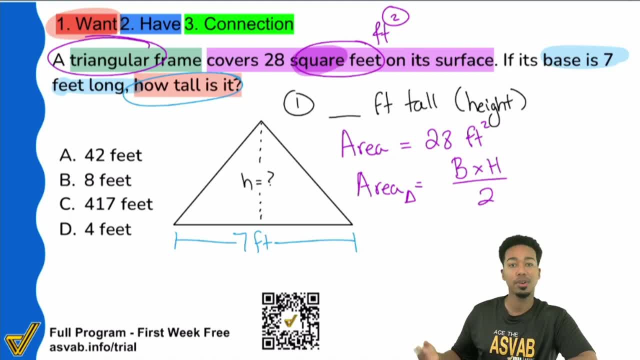 And we are given the area as, again, 28 square feet. So all we're going to do here is we're going to plug in the information and we're going to have ourselves a good time. That's it, The area that we're given. my party people will remember that was 28.. 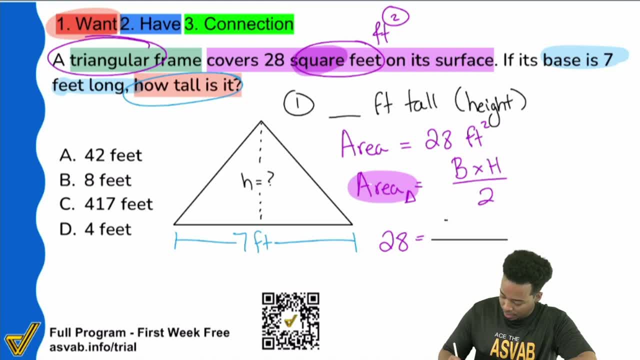 Then the base that we were given was seven, And then we're looking for the height, And then we are filling in the rest of the formula. Now, all I have to do, my party people, all I got to do is go ahead and solve this equation here And 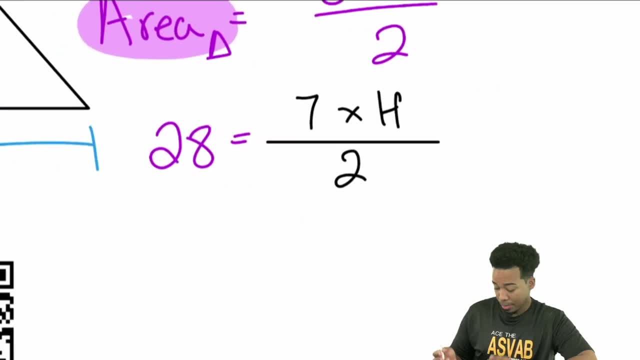 we're set, Here we go. First things first. I could probably get away with multiplying both sides by two, Or you could divide both sides by seven. Either way, you're just trying to get rid of everything around the H, right there. So again, like I said, we can multiply both sides by two. 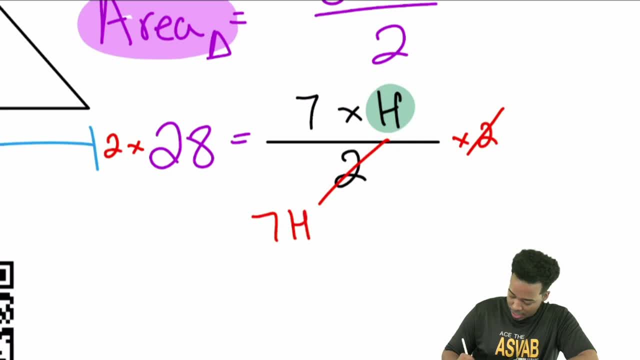 To get rid of that entire denominator so that we can have seven. H equals 28 times two, which would give us 56. It's very wise to know your mental math to be able to do stuff like that in your head, because saves you time Next up. And lastly, we would divide both sides by seven And 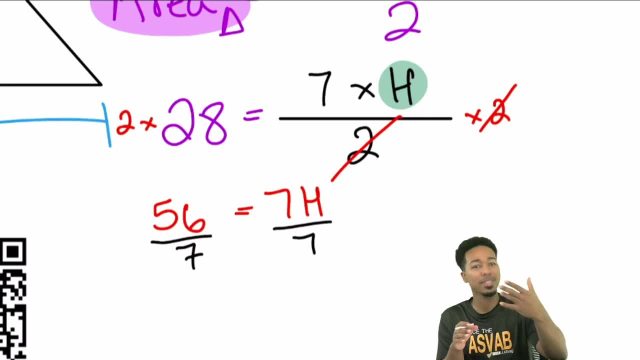 before I say the final answer, remember, if you like this video, go ahead and leave a comment like this video and subscribe to the channel. You know how much it helps us out And we know how much we are excited to really help you out, So I want you to be as excited for us as we are about 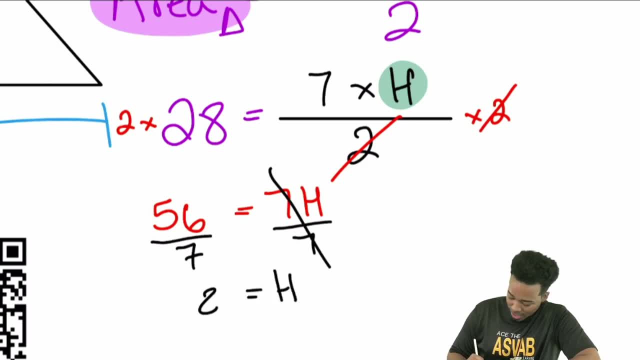 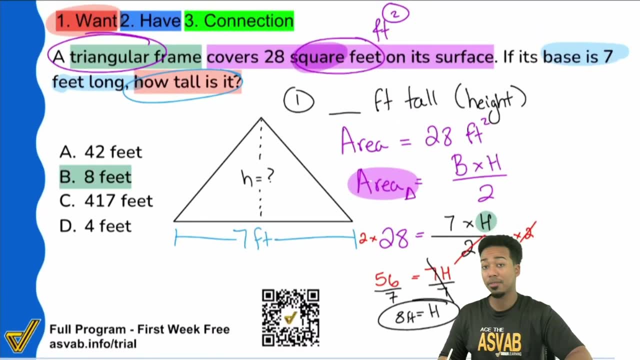 the answer here? The answer here will be H equals eight and it'll be eight feet. And there it is my party people. The answer is B, eight feet. And remember that if you want to practice literally thousands upon thousands of problems just like this, with step by step written explanations, 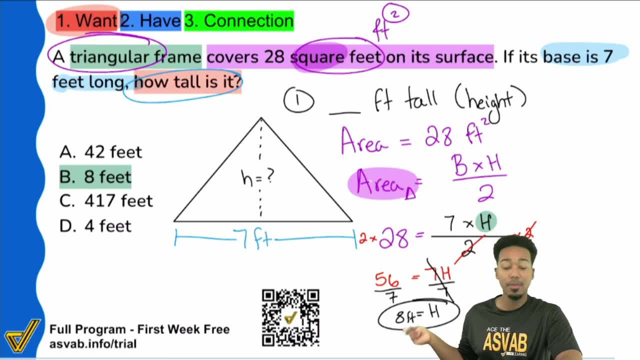 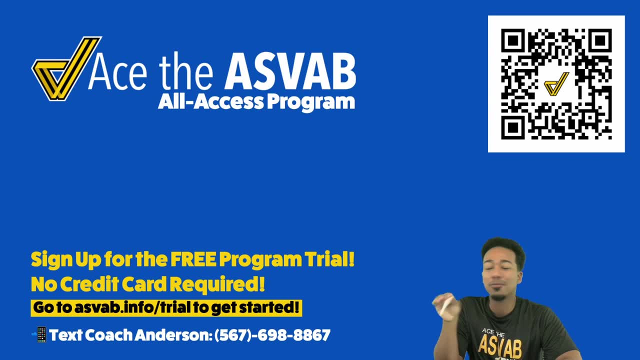 we got your back because we have everything you need in our full program And that's going to be located right there at that QR code or this QR code right here. We're excited to help you guys out. Our full program is free for a full week, No credit card required. Get in that.